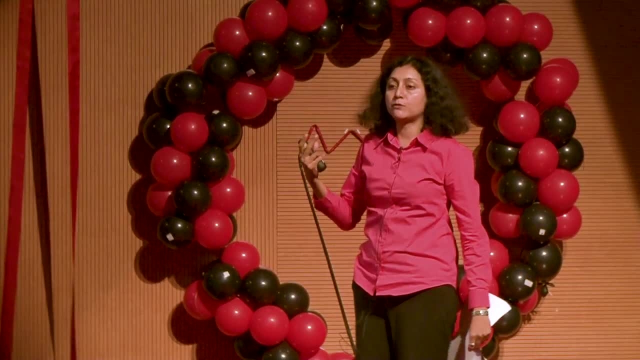 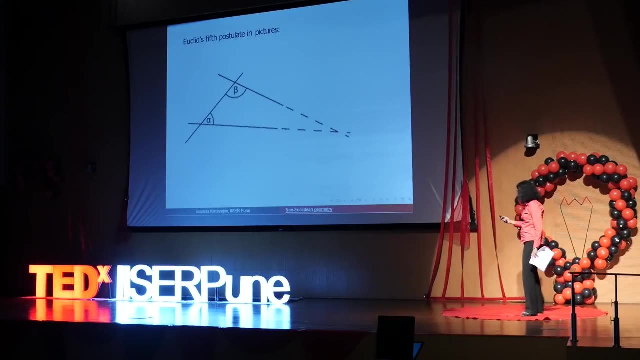 line. Rule number three talks about what are circles, Rule number four talks about what are right angles, And rule number five is a little bit complicated, So I'm going to show you in figures. There are two straight lines here and there is a third line which 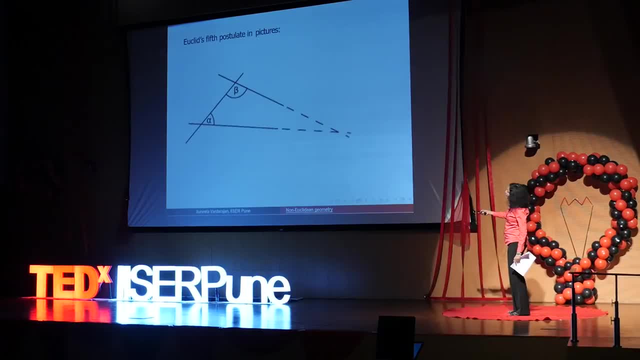 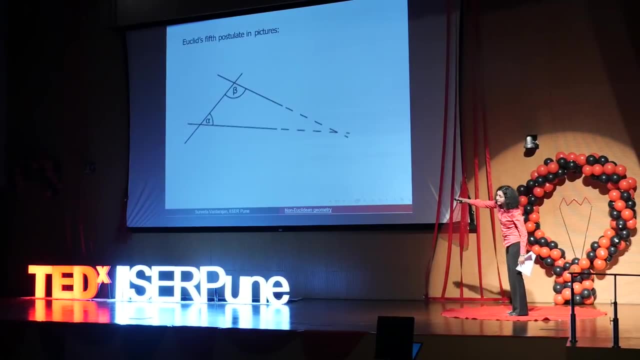 intersects them and you see two angles: alpha and beta. okay, If the sum of the two angles is less than 180 degrees, then the two lines meet on that side. So they don't meet on the other side, They meet on this side because the sum of the two angles is less than 180. 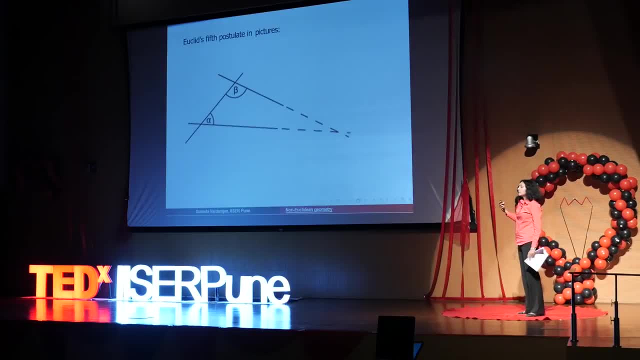 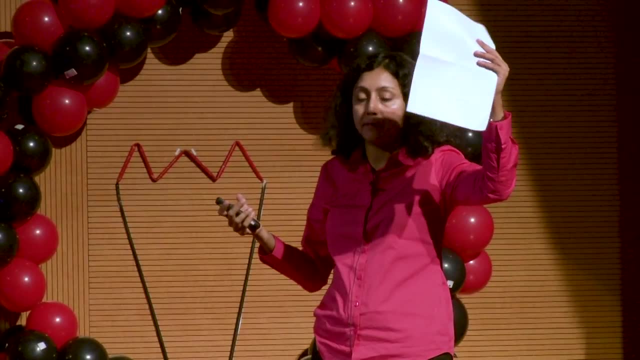 degrees. This is Euclid's fifth rule. Now, these rules, as you can guess, did not come from his imagination. They are obvious experiments that you can do on a piece of paper with a pen. okay, So you can just draw these things and you would immediately know that these 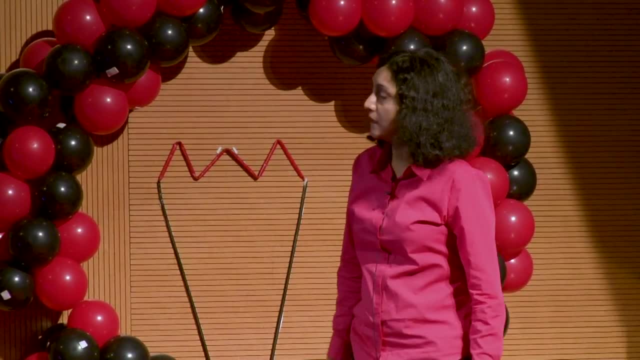 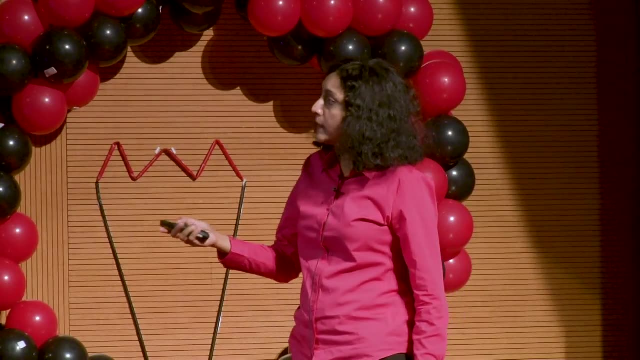 rules are obvious. Now there's another way of stating this fifth rule, which is very popular. It's called the parallel postulate. Postulate is just a rule. Now what it says is that you take one point, You take a point, You take a point, You take a point, You take. 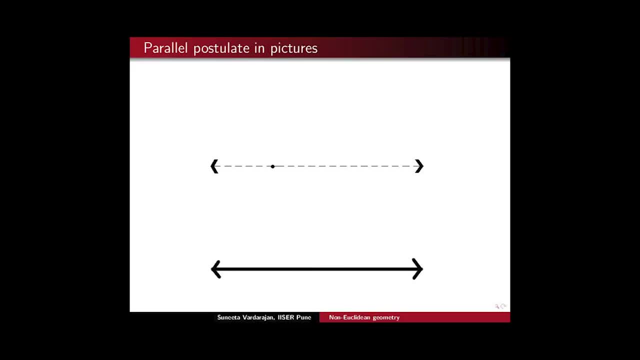 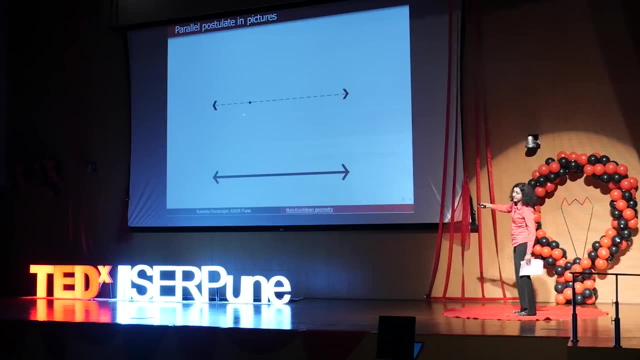 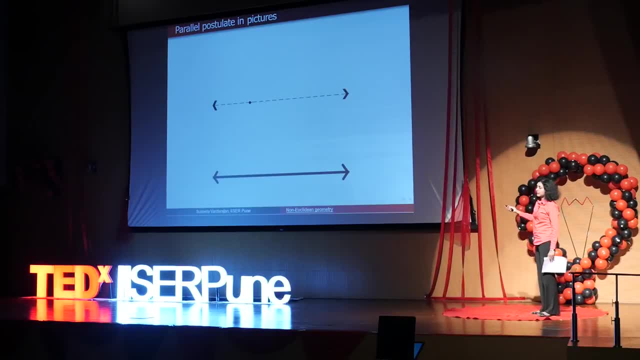 line. okay, That's what the rule says, and that is completely equivalent to the fifth rule, which I stated before. The proof is long, okay. So here are Euclid's five rules, and these five rules define the geometry that we learned in elementary and middle school. 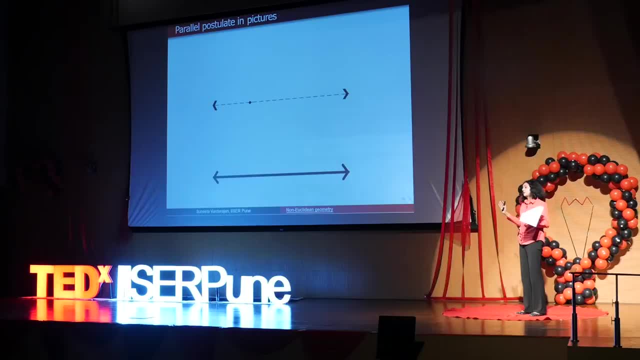 It's called Euclidean geometry. We view the whole world from that perspective. okay, But then a lot of people asked what would happen if we dropped one of these rules? okay, Would our familiar school geometry still follow? And then, quickly, the German mathematician Gauss realized: 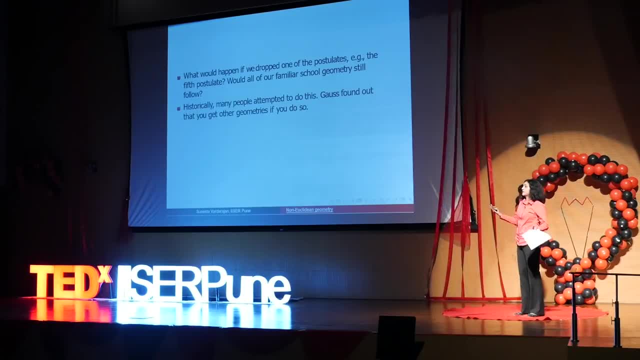 that our school geometry will not follow. if we dropped, for example, the fifth rule, okay. If we said, the fifth rule is not valid, then we would get other geometries. if we do so, okay. Now what do I mean by other geometries? 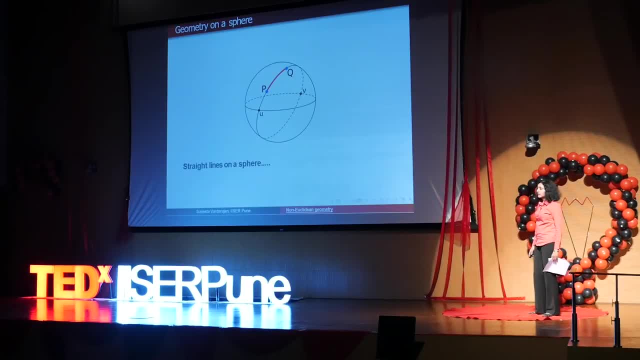 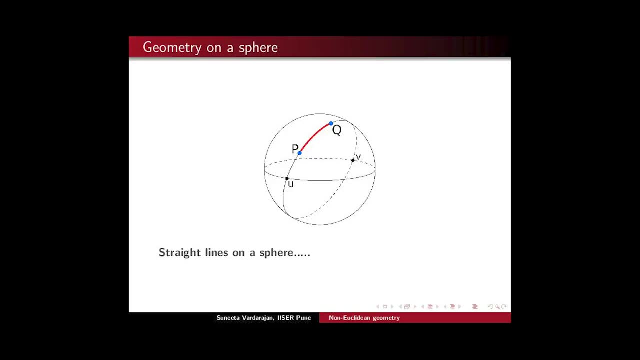 So what I mean by other geometries, to give you an example, is this geometry on the surface of a ball. So you take a big basketball or something and the surface of the ball is a sphere On that geometry. imagine that there are two points. 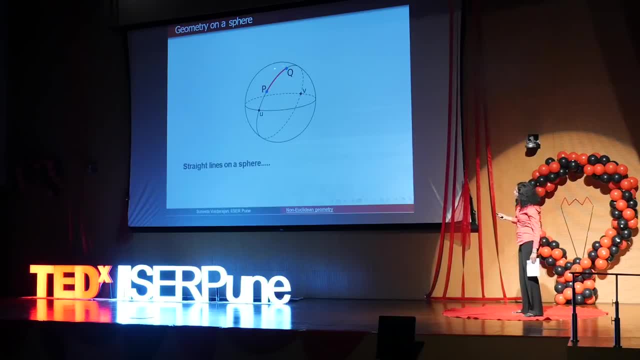 P and Q okay, And I'm looking for the path of shortest distance between those two points. Imagine there's an ant and the ant is crawling on the sphere and it wants the path of shortest distance between the points P and Q. 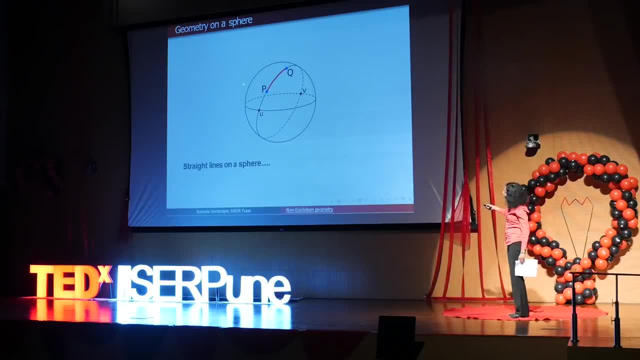 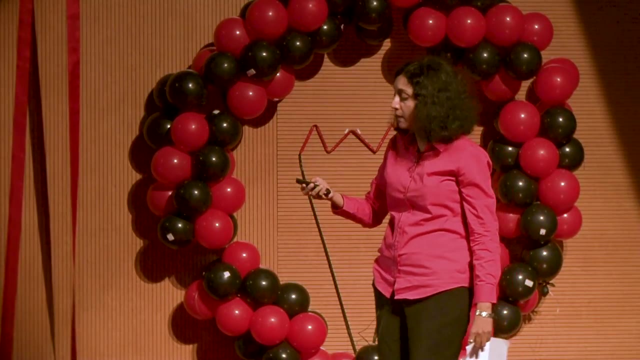 What would that path be? That path would be the arc of this circle. okay, This is called a great circle because this circle has as its diameter the diameter of the sphere. So the path of shortest distance looks curved to us from our perspective of Euclidean geometry. okay, 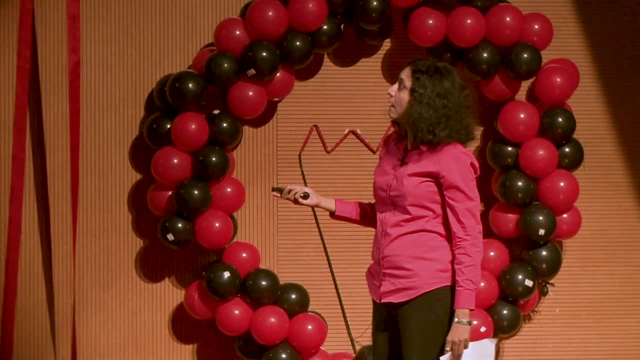 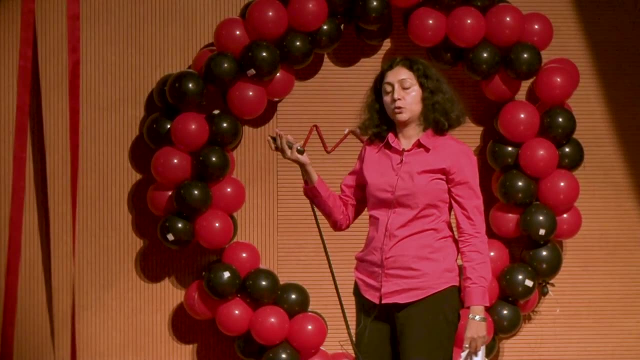 And it's this arc of a great circle, And airline pilots know this all the time, right When they are. when you're traveling from one part of the world to another, you have to go through the path of shortest distance, and that's what they are doing all the time. 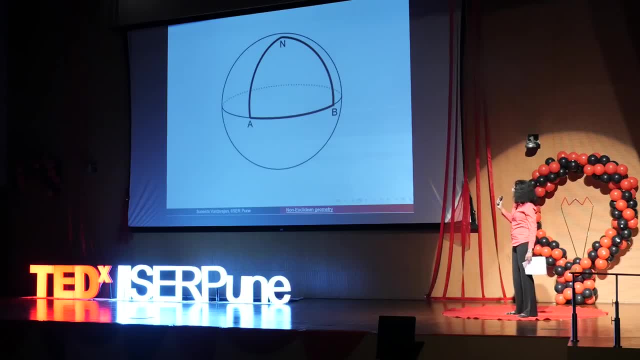 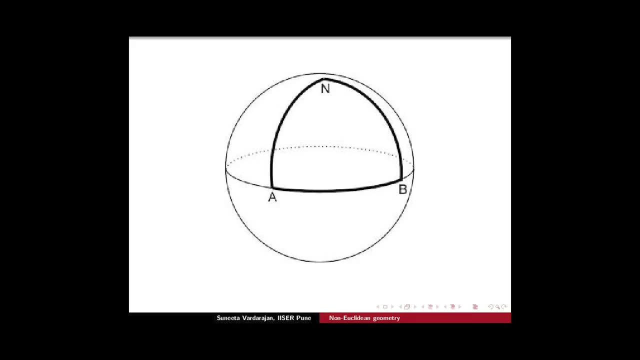 Now let's come to the next figure, which looks a little bit to everyone like a triangle. but it doesn't look quite like a triangle, because what is a triangle? A triangle is on the sheet of paper I will draw, put three points. 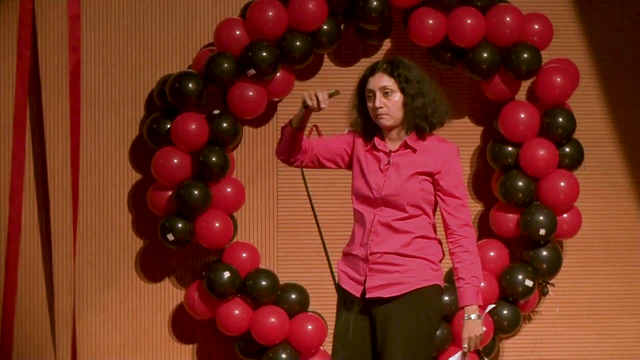 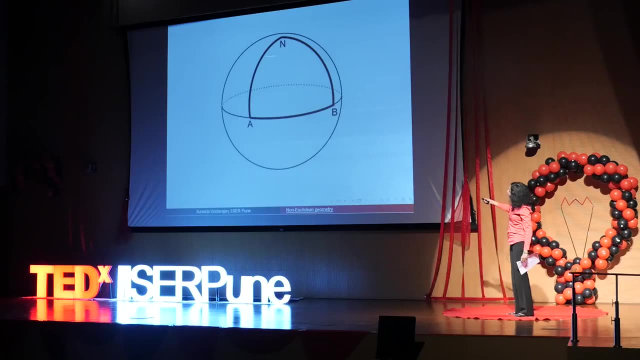 which are not on the straight line on the same straight line and I will connect them by lines. That would be a triangle. okay, That's exactly what I've done here. I've taken three points on the sphere N, A and B. 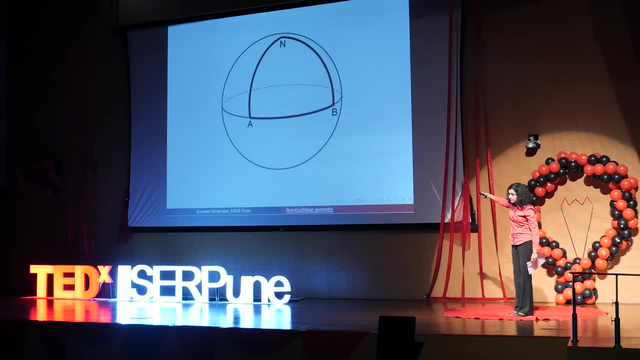 and I've connected them using what are straight lines on the sphere. Those straight lines are these arcs of circles, okay, And I formed this triangle. Now you can easily see that the sum of the three angles of this triangle should have been 180 degrees. 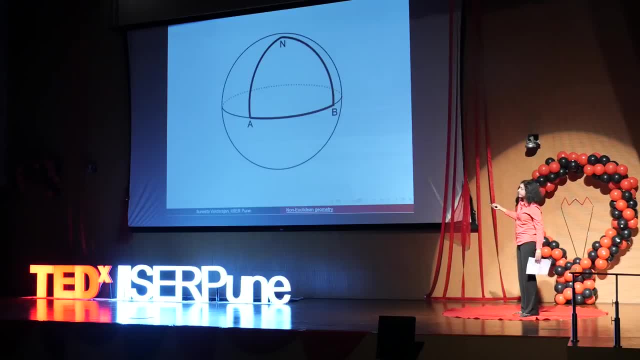 if you remember your elementary school. but it's not 180 degrees here, It's much more than that. okay, This is called a spherical triangle, And if you look at the line that starts from A and the line that starts from B, 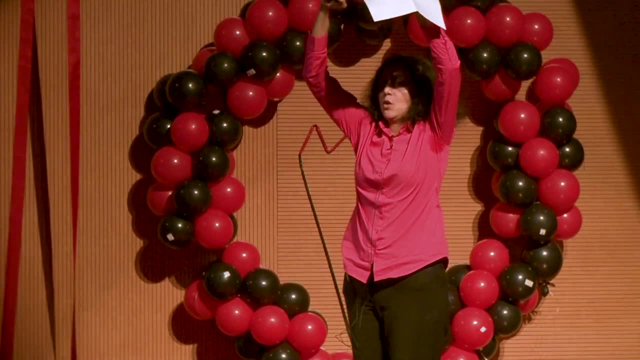 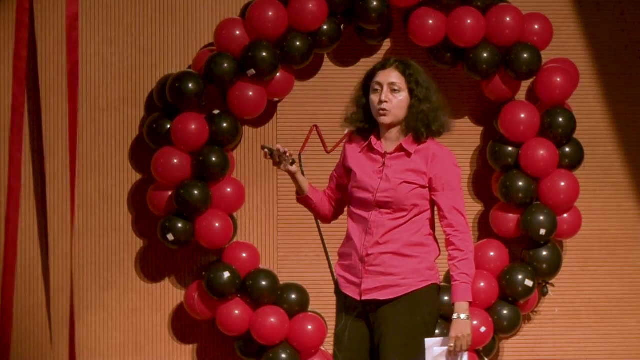 they start out looking parallel initially, but then they meet okay. So because they meet, there are no parallel lines on the sphere, So there is no fifth rule of Euclid on the sphere. There's no question of talking about one line being parallel to another. 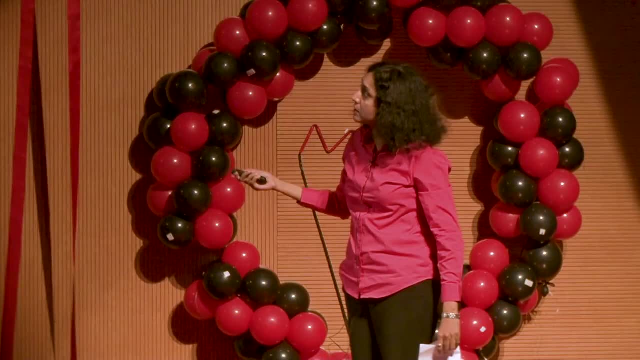 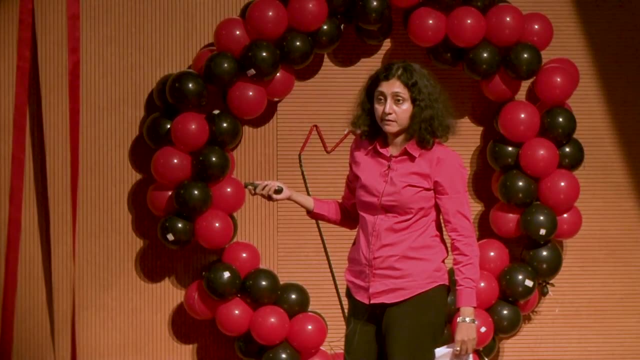 because there are no parallel lines on the sphere. okay, So this sphere does not obey Euclid's fifth rule. And on this sphere, the sum of the three angles of a triangle is not 180 degrees. It is much more than that. 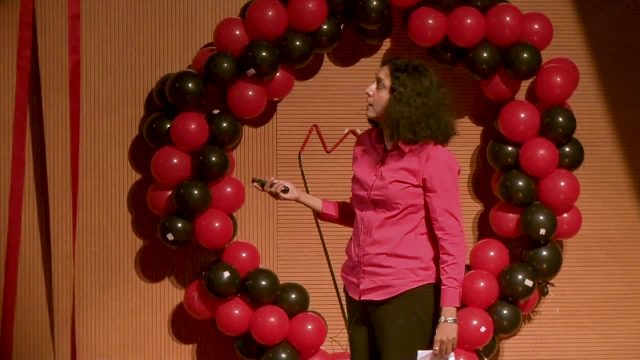 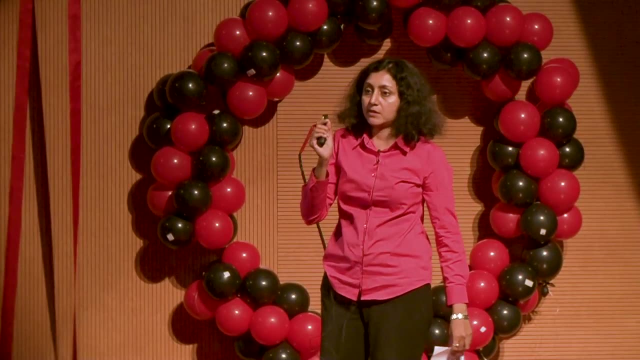 So we've dropped our elementary school geometry. It is much more than that, by going on the sphere. So there's one more thing that we can do, one more experiment which captures the geometry of the sphere and which tells you that it's different from that of this sheet of paper. okay, 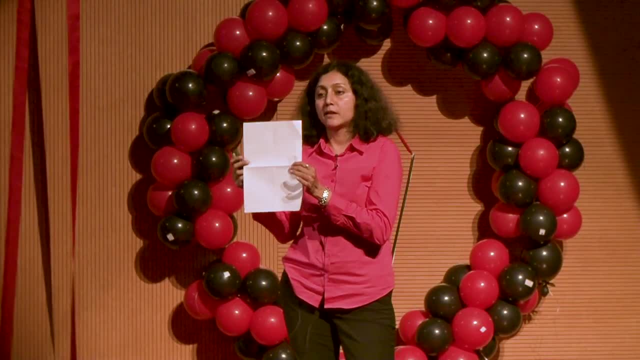 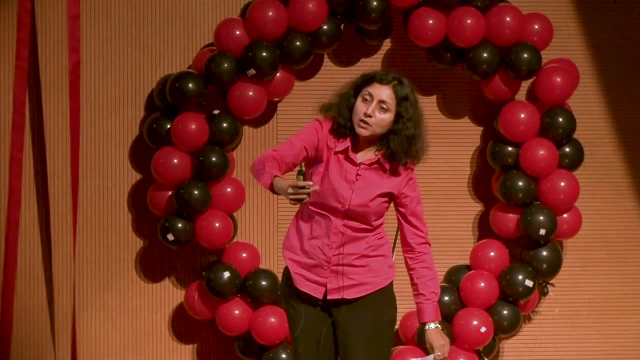 Now, what is that? Now, on this sheet of paper, I can draw circles. I can draw a big circle, I can draw a small circle. The ratio of the circumference, which is the length along the circle, to the radius, will always be the number two pi. 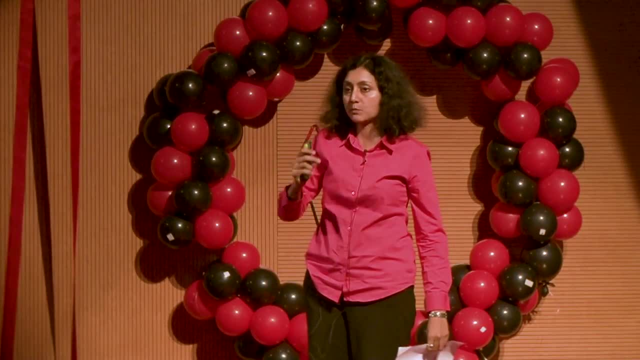 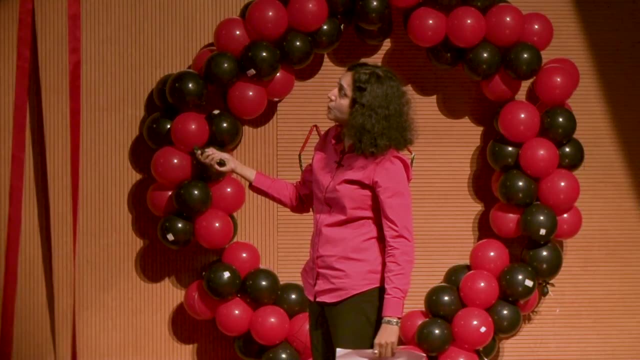 no matter what is the size of the circle. It could be big, it could be small. That ratio will always be two pi. the number two pi Now on a sphere. imagine an ant. This ant is walking along the radius. 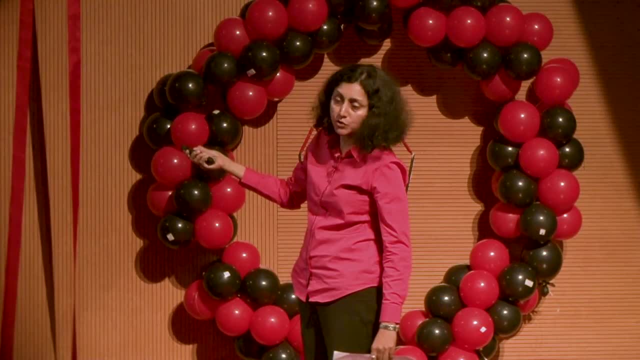 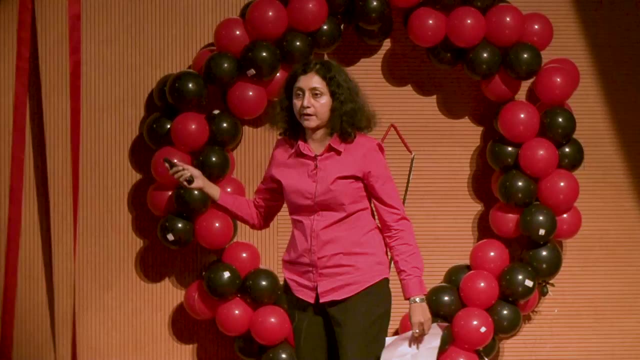 This is the radius: by being on the sphere, Remember- the ant cannot cut through the sphere right, So it's walking along the sphere and then it covers the circle, and the ratio of the circumference to the radius will not be two pi. I leave it to you to think about. 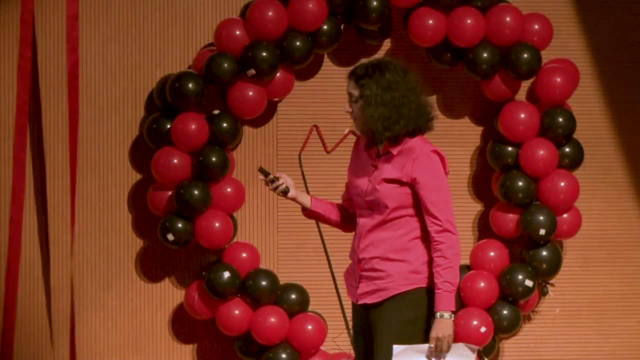 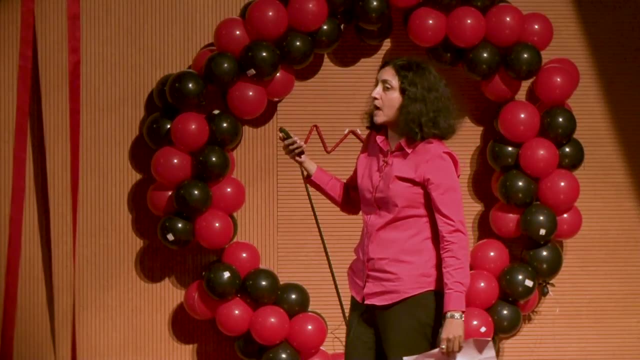 whether it would be less than two pi or greater than two pi. Okay, So this experiment also captures the different geometry of the sphere. So this is what I mean by other geometries. Now, the realization that we come to is that, by dropping the fifth rule, 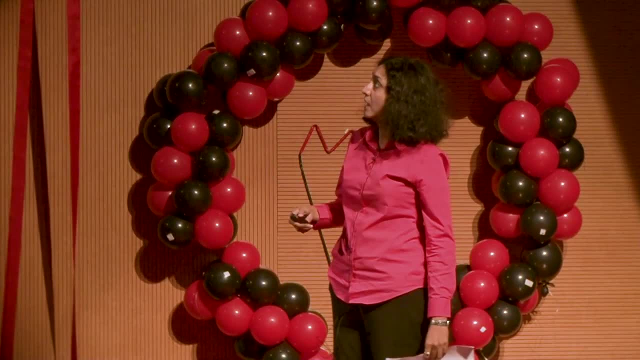 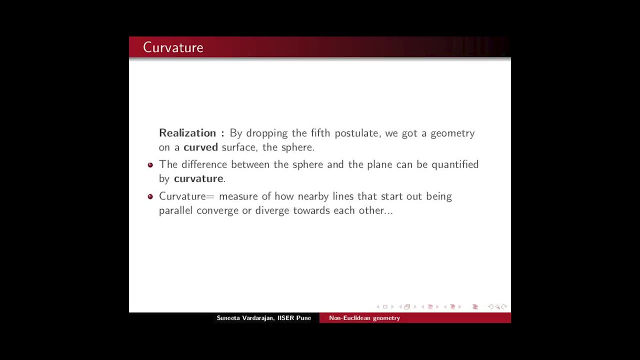 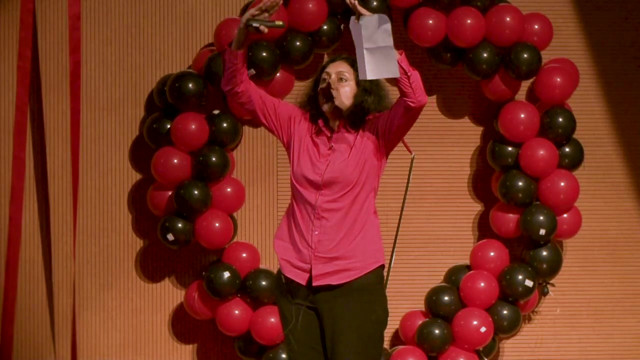 we got a geometry on a curved space, which is the sphere. The difference between the sphere and this plain sheet of paper can be quantified by something called curvature. Now, what is curvature? It's a measure of how nearby lines that start out being parallel converge. 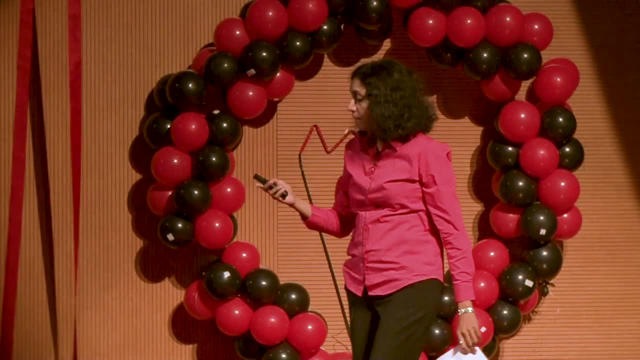 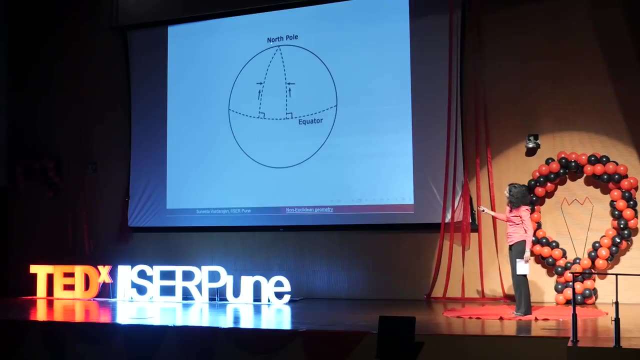 or diverge from each other because of curvature. So here's an example of the sphere. again, Here are two lines that start out looking parallel to each other, but then they eventually meet at the North Pole and they converge. they converge because of curvature. 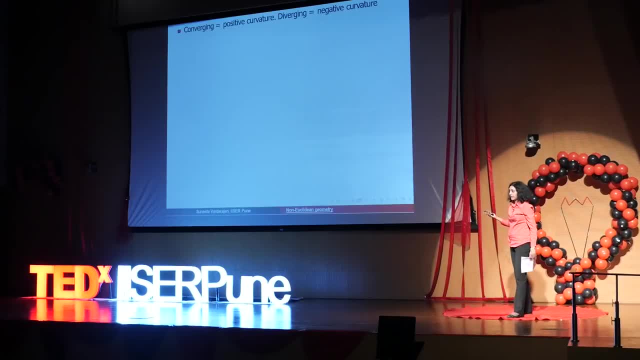 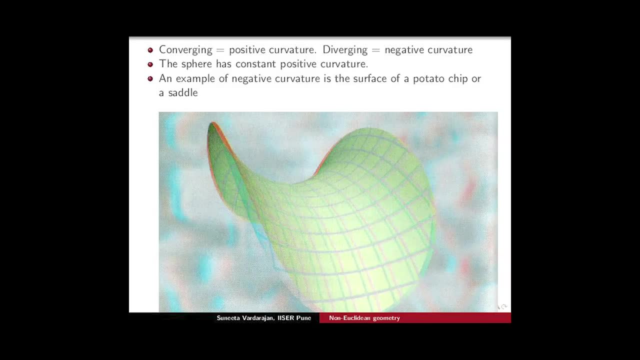 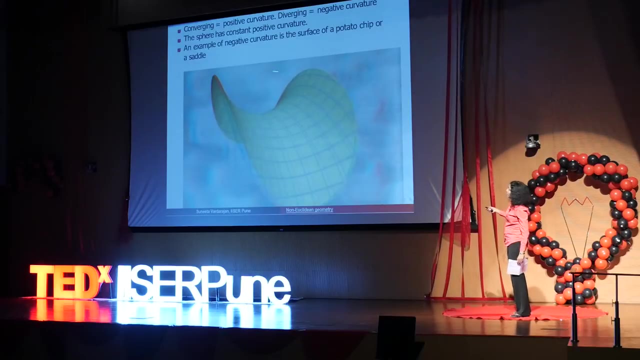 Now, converging is positive curvature and diverging is negative curvature. The sphere has constant positive curvature And here's an example of a negative curvature surface, Which could be the surface of a potato chip or of a saddle. Okay, this is an example of negative curvature surface. 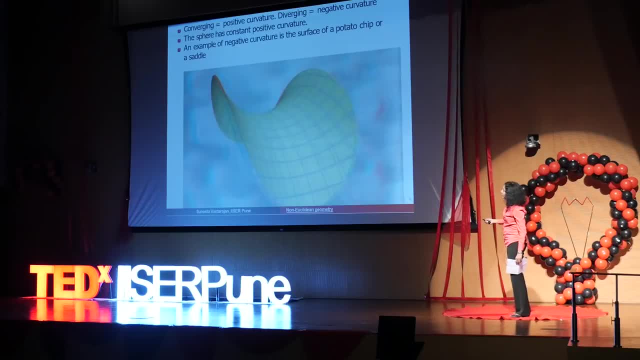 If an ant were to move on this negative curvature surface, it would discover that the geometry is very different from that of the sphere. Now geometers: mathematicians of the 19th century such as Bolyai, Lobachevsky and Gauss. 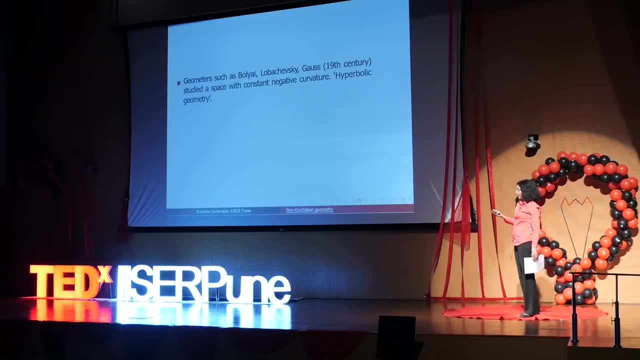 studied a space with constant negative curvature called hyperbolic geometry. Now, this I absolutely need to mention for historical reasons, This is a geometry which is best visualized on pen and paper, but it was historically very important that they. what they did was they dropped this fifth rule of Euclid. 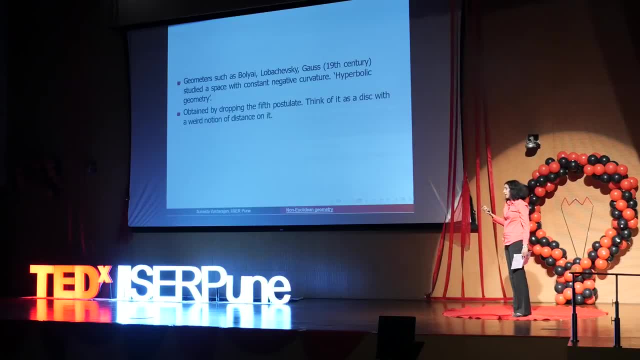 and then they got this geometry. Okay, so the sphere is not the only geometry you get when you drop the fifth rule. you can also get this geometry. Now you can think of this as a disc with a weird notion of distance on it. 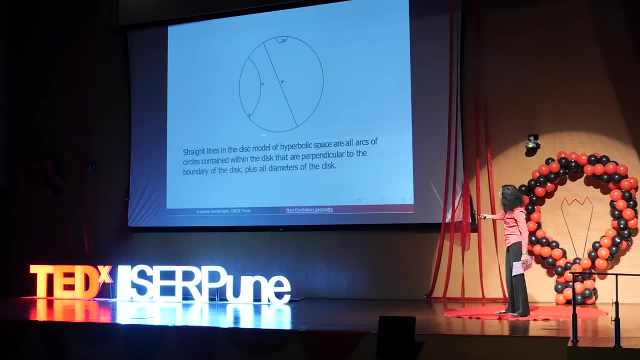 So let me explain to you. this is a disc, Okay, it has a weird notion of distance. according to that notion of distance, the paths of shortest distance or the straight lines are like this: They are these kind of circles which meet at 90 degrees. 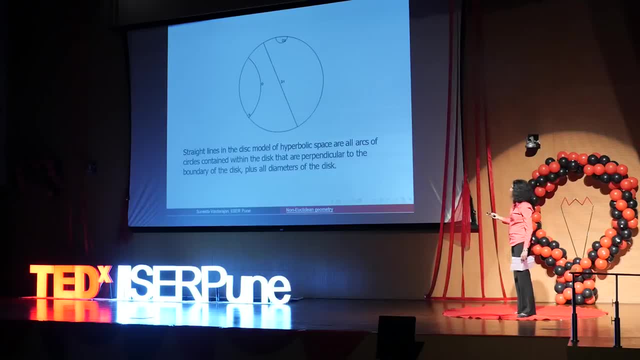 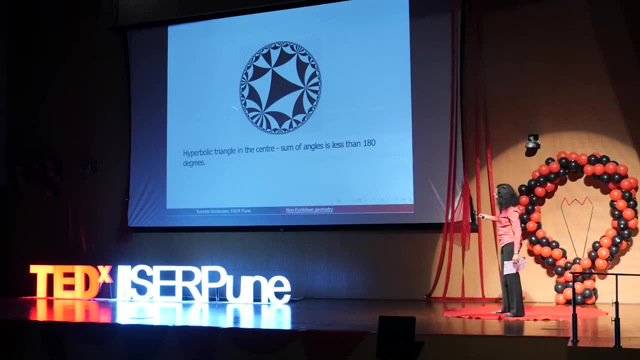 or the diameters of the disc. This is hyperbolic geometry. Okay, this is a geometry that you get by dropping the fifth rule of Euclid. Now here is an example of triangles in this geometry. See these lines which join the three points together. 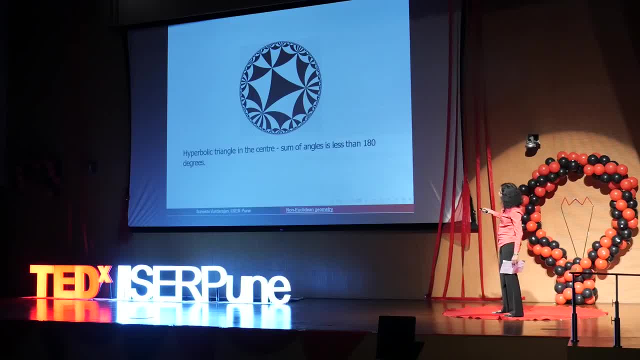 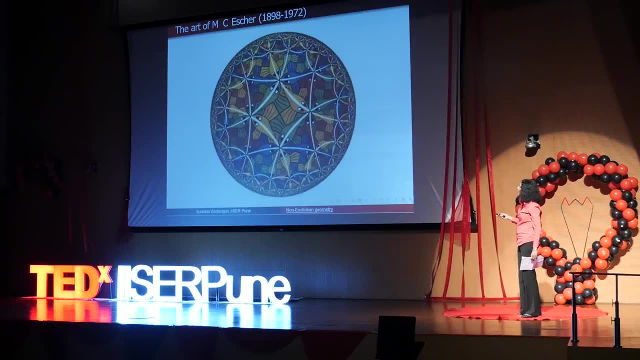 they are actually straight lines in this weird geometry, with this weird notion of distance, And the sum of the three angles of a triangle here is less than 180 degrees, because the space has negative curvature. And here's a beautiful artwork by the Dutch graphic artist MC Escher. 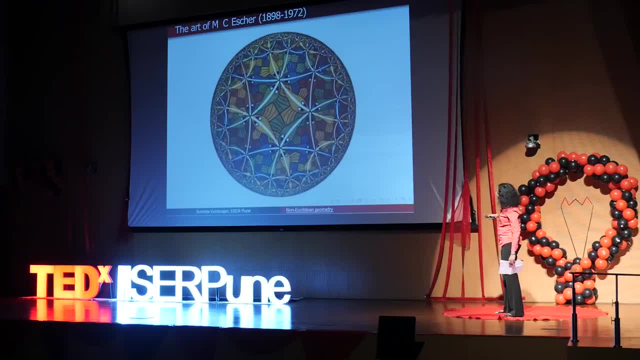 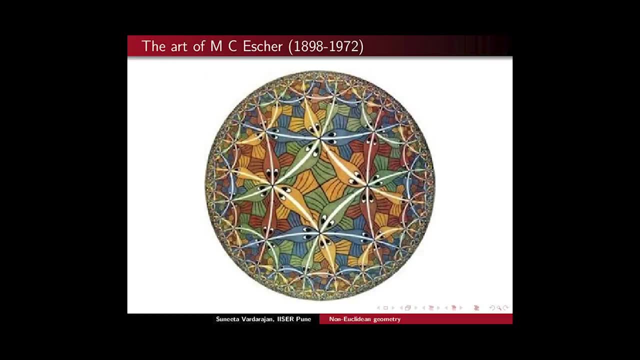 What Escher did was he knew hyperbolic geometry, and so he took what are lines in hyperbolic geometry, which are these curves, and he drew fish along those curves. Okay, so you have all these fish moving along curves which are like straight lines in this hyperbolic geometry. 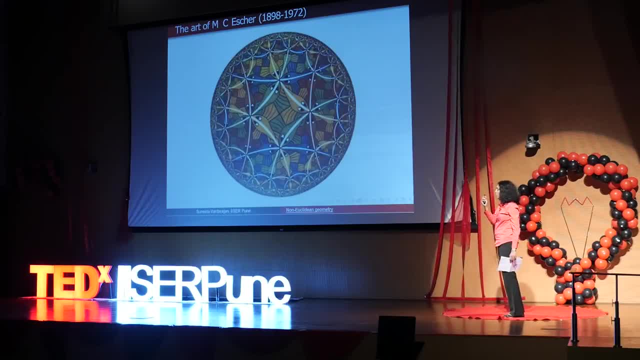 And to us from the perspective of Euclidean geometry, the geometry that we learned in school. all these fish are of different size, but with the weird notion of distance and hyperbolic geometry, these fish are all of the same size. So these are some examples of another geometry. 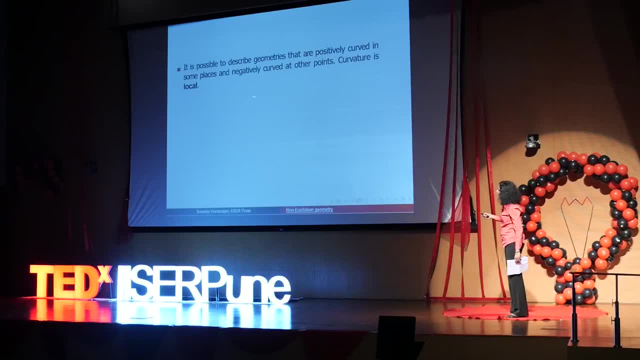 Now it is possible to describe geometries that are positively curved in some places and negatively curved at other points. Curvature is something which is local, and these will be the natural geometries on different curved surfaces. So, for example, if I look at this: 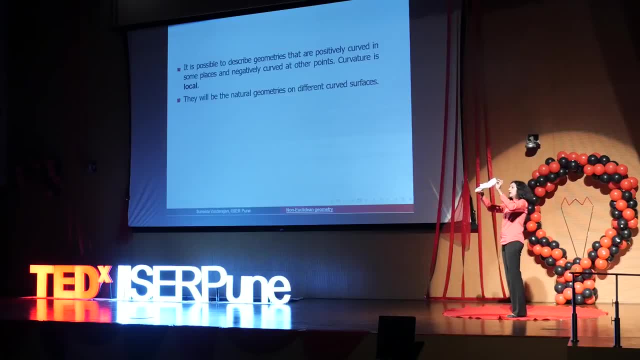 have. if I crumple this piece of paper, I have a curved surface. At some points, the geometry will be such that there is negative curvature. at some points, the geometry will be such that there is positive curvature. Now I want to slightly change tracks and I 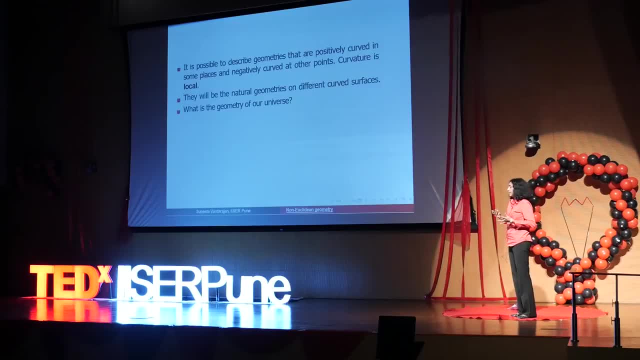 want to ask a question, which I'm asking because I'm basically a physicist: What is the geometry of our universe? And I want to connect all that we have studied so far- which is like a mathematical curiosity- to the geometry of our universe. So why suddenly talk about this? 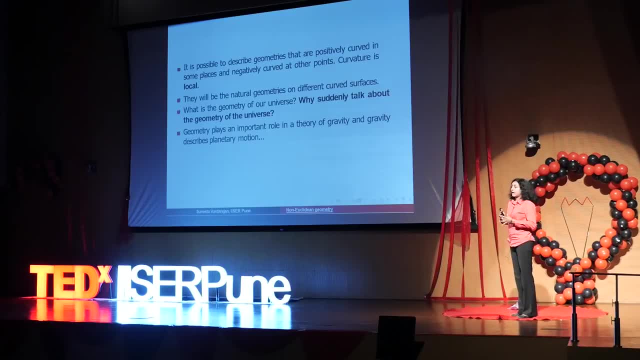 The reason is that geometry plays a role in a theory of gravity, and gravity describes lots of things that are going on in the universe. For example, gravity describes planetary motion. Now, what is the geometry, What is the theory of gravity that we have learned in school? 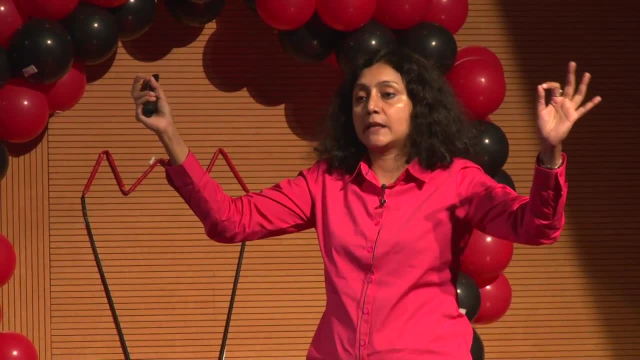 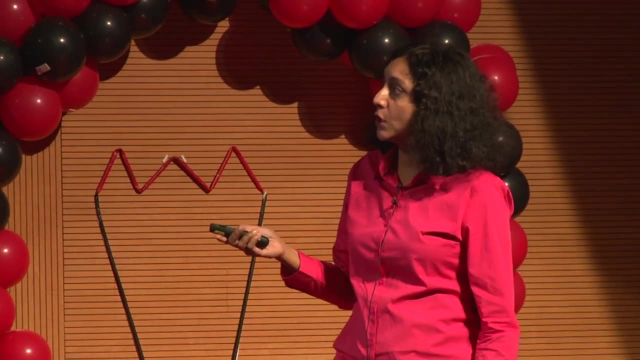 We have learned about Newton's theory of gravity, which tells you that any two massive objects attract each other with a force. Okay, This was replaced by Einstein by a theory of gravity in which gravity is not a force. It is not a force between masses, as Newton thought. 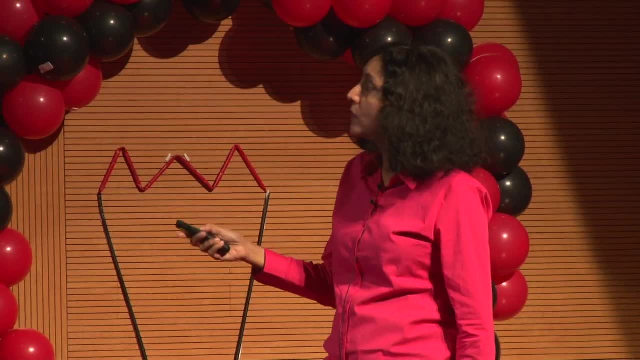 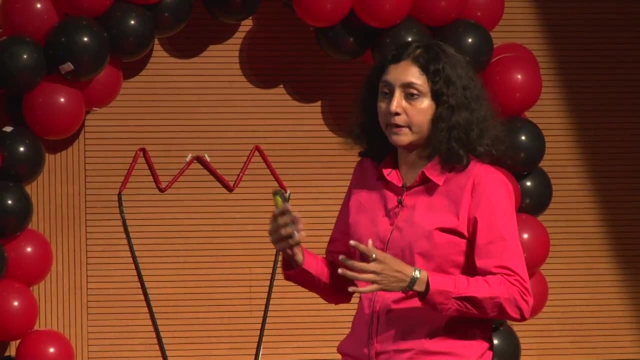 This is Einstein's theory of gravity in 1915 and gravity is actually the geometry. It's geometry of space, and not just space but space and time. That's a little bit complicated to explain. But gravity- you can think of gravity as the geometry of space. 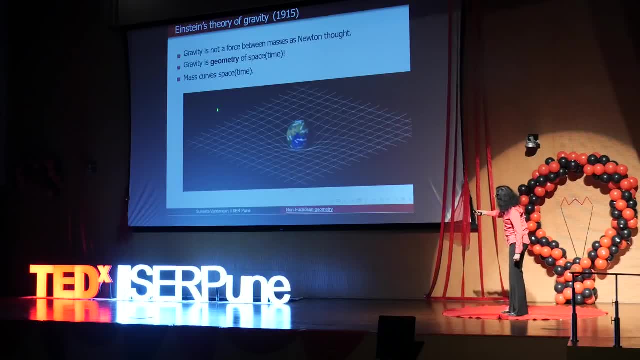 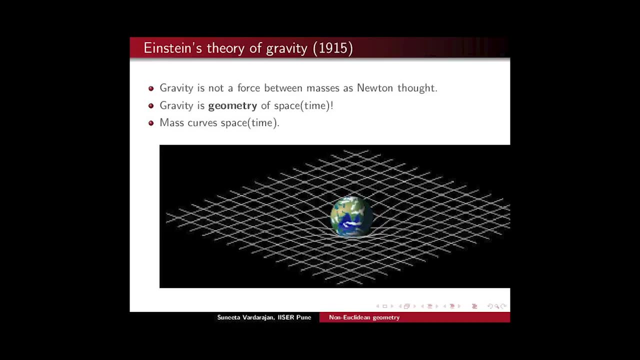 What mass does? what any massive object does is that it curves the space and time around it. So imagine that you have a rubber sheet and you have some really massive ball. The ball is placed on the rubber sheet. The ball deforms the rubber sheet. 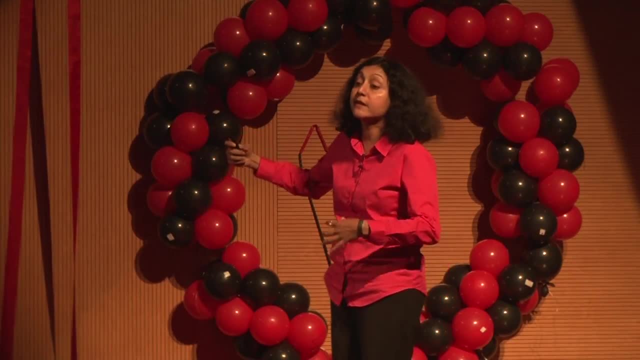 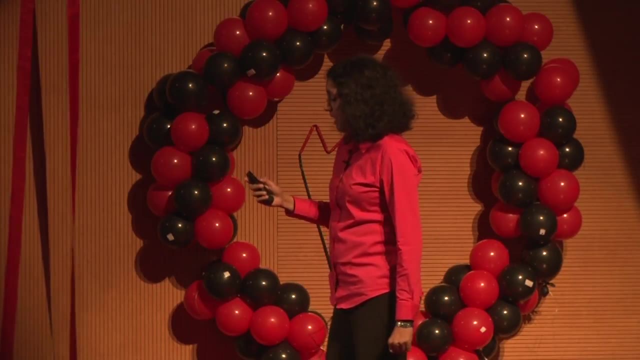 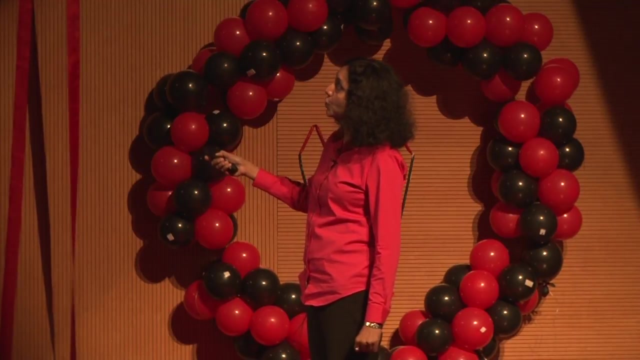 In the same way, the mass deforms the space time around it. It creates curvature, So it makes the geometry different from the Euclidean geometry. And here's a picture which I want you to follow with me. This is a drastic, You know, experiment which shows you that matter curves geometry.